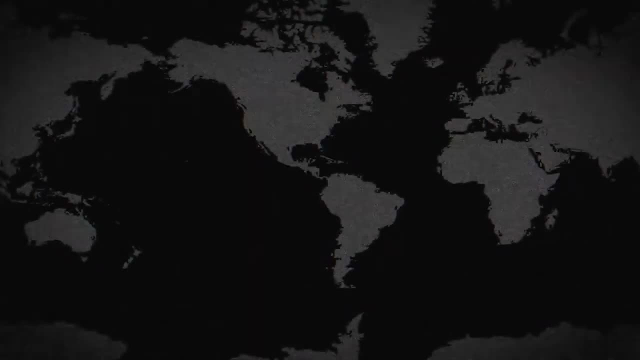 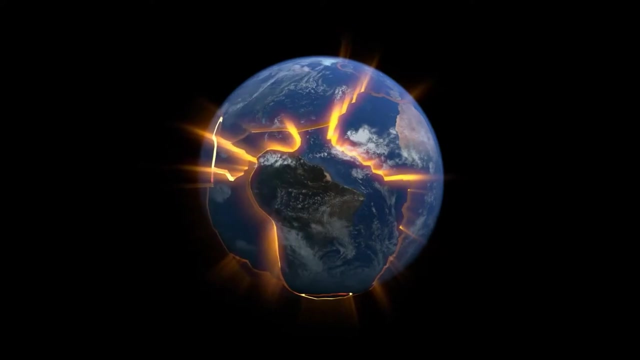 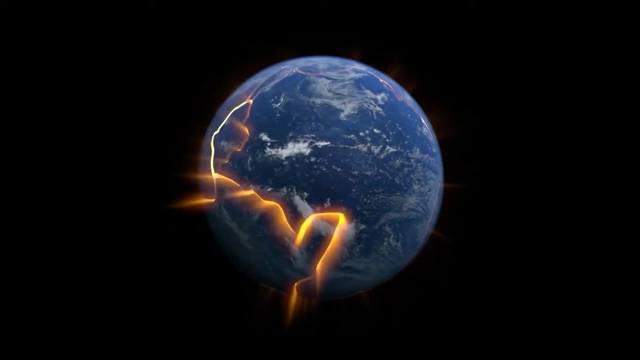 Our last hazards video ended with us saying: as you'll see in our next video, the real action happens along the edges of the tectonic plates. So now it's time to take a look at plate boundaries, sometimes also called plate margins, which are all of the parts of the world where one tectonic plate is next to. 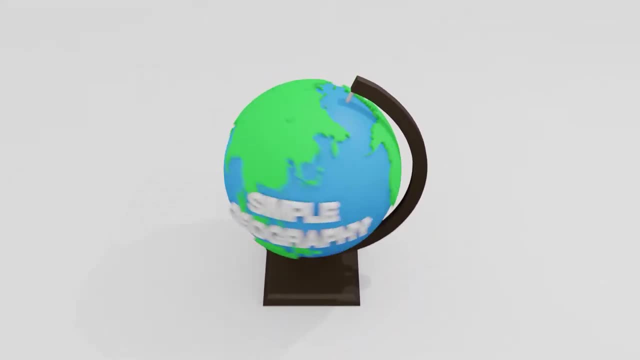 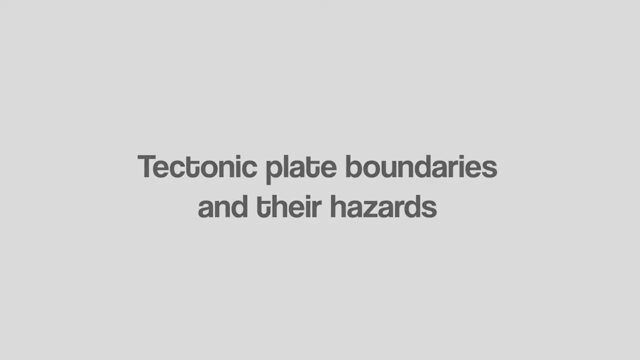 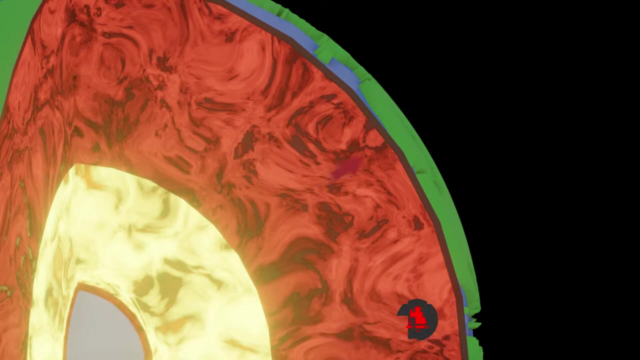 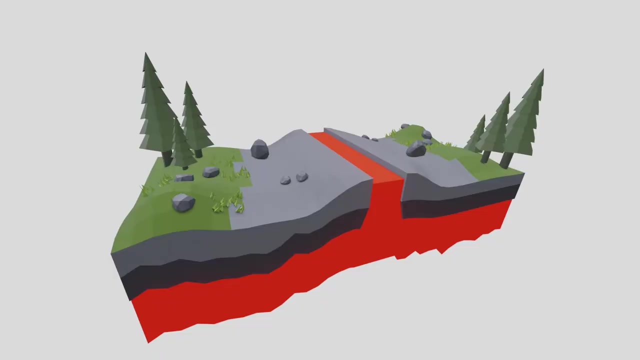 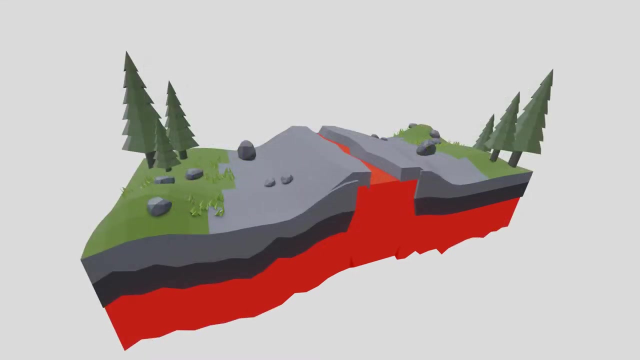 another Constructive, sometimes also called divergent plate boundaries exist in the parts of the world where magma is rising up in the mantle. below This rising magma cools off and spreads out. Some of it solidifies and creates new crust which begins to slowly move apart as two separate tectonic plates. These types of 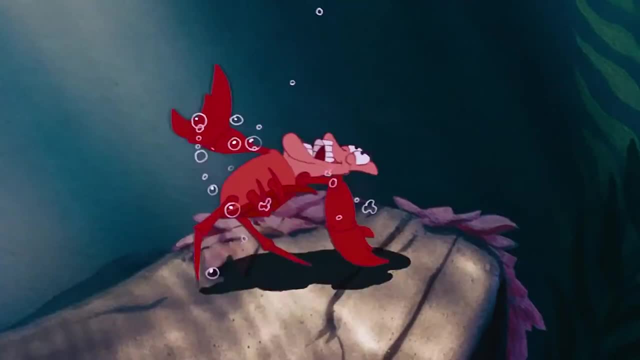 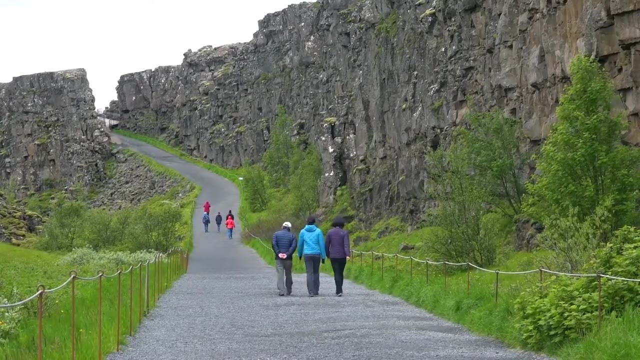 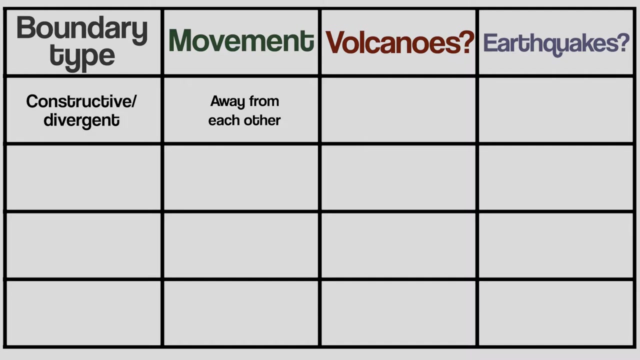 boundary mostly appear at the bottom of the sea. There are some places, like Iceland, where you can actually see evidence on land of the tectonic plates splitting apart. So what type of hazards do we find here and why? Let's start with volcanoes. Some of 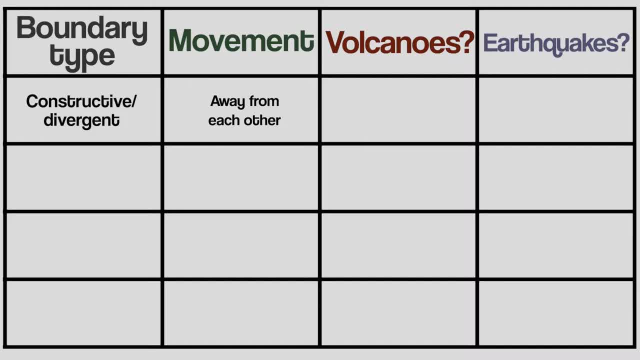 the magma, along with gases like carbon dioxide, can melt through the crust and get released out of the surface, which is basically what a volcanic eruption is. So, yeah, we get volcanoes, Often with lots of lava. Earthquakes do happen at constructive boundaries, but 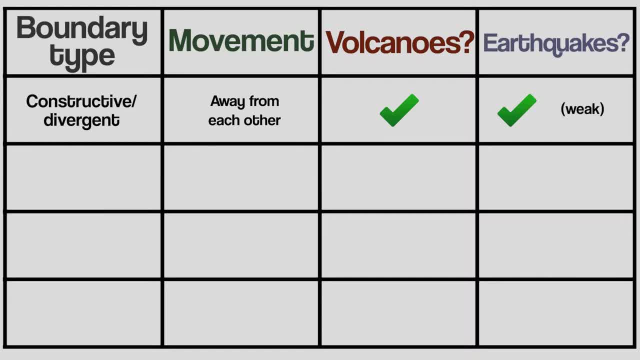 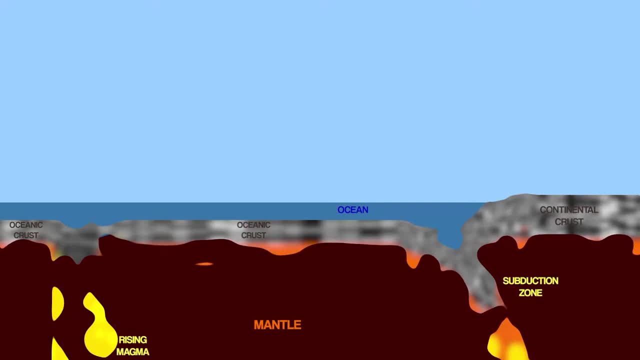 they aren't usually that powerful. You see, an earthquake happens when tectonic plates get stuck or grind against each other. It just doesn't happen very much at this kind of boundary because the plates are mostly moving apart. Destructive, sometimes also called convergent boundaries are areas where 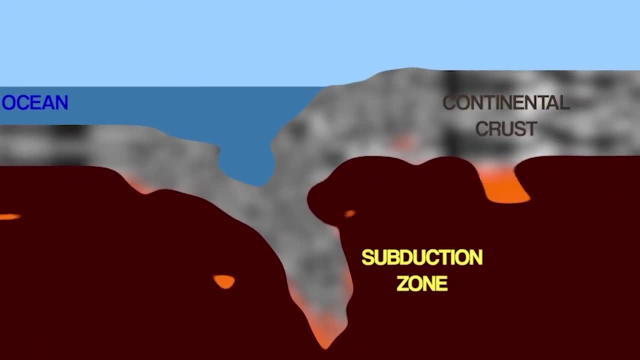 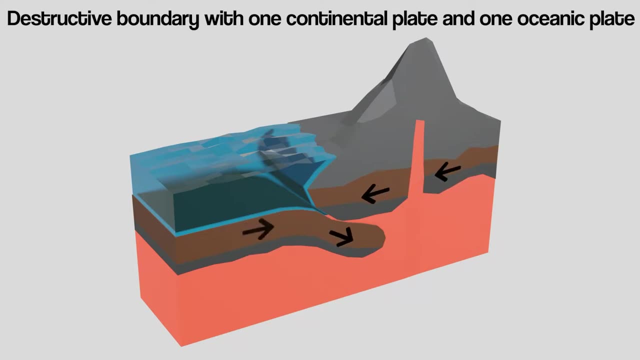 tectonic plates are being carried towards each other, but there are a lot of them. There are actually two different types. If an oceanic plate is moving towards a continental plate, the oceanic plate is forced underneath because it is denser in a process we call subduction, As the oceanic plate sinks into the mantle water. 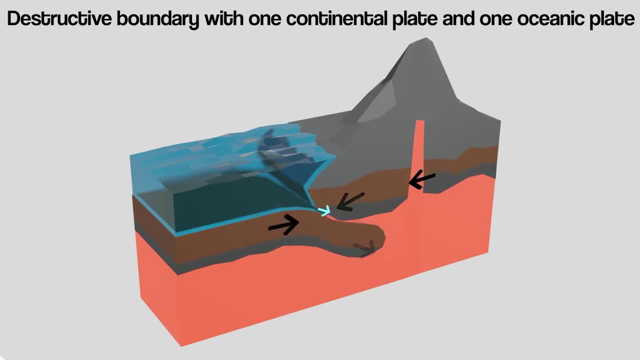 and things like dead plankton on the seafloor are dragged down with it. These are turned into water vapor and carbon dioxide, which bubble upwards and melt through the continental crust above and get trapped in the rock. Pressure begins to build up much like it does when you shake a bottle of vodka. If you shake a bottle of vodka, the pressure begins to build up much like it does when you shake a bottle of vodka. 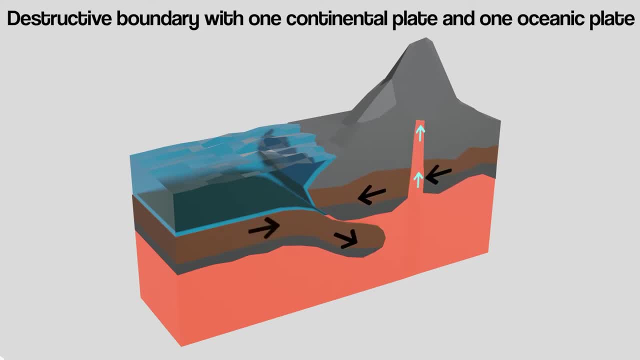 drink and eventually the pressure in the crust becomes too great and the gas and lava violently explode out of the rock in a volcanic eruption. Extremely powerful earthquakes can also happen at these destructive boundaries. The oceanic crust doesn't simply slide gently past the continental plate. These 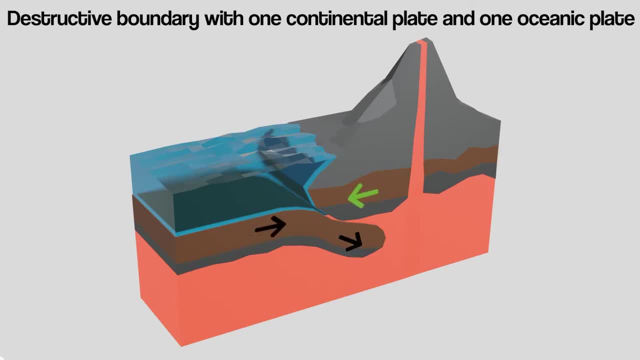 huge rough slabs of rock are constantly grinding against and getting stuck in each other. and when they do get stuck, the continental plate starts getting dragged down. with the oceanic plate It builds up a huge amount of energy as this happens. When the plates finally become unstuck, the plate 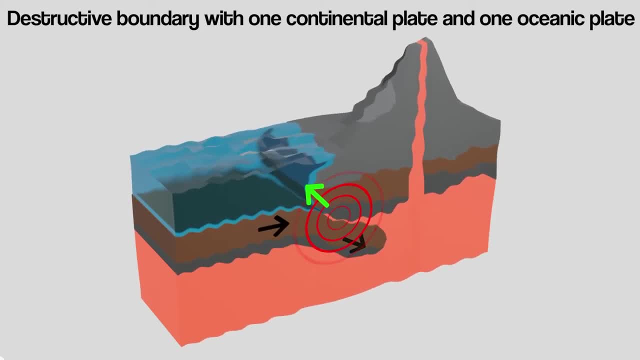 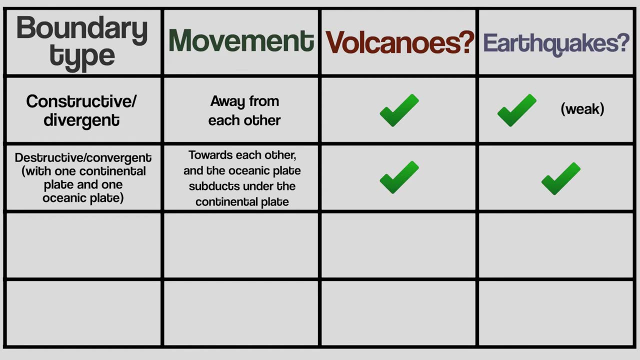 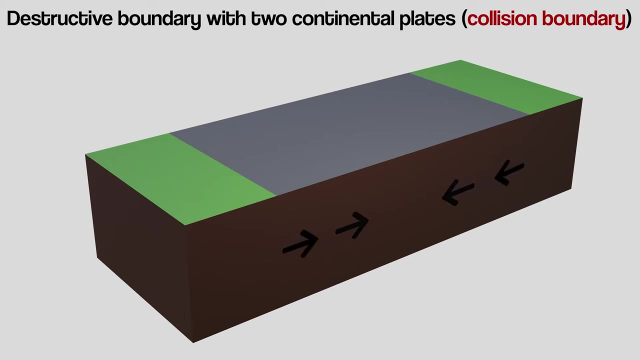 violently jumps upwards, releasing all of the stored energy and causing intense shaking in the ground. We know this as an earthquake. The second type of destructive plate boundary is known as a collision boundary. The big difference here is that both of the tectonic plates are continental, so they have roughly the 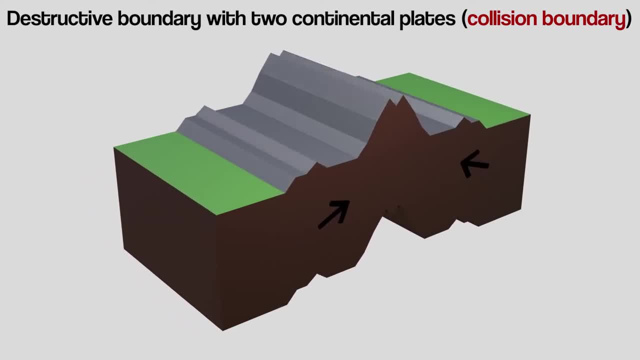 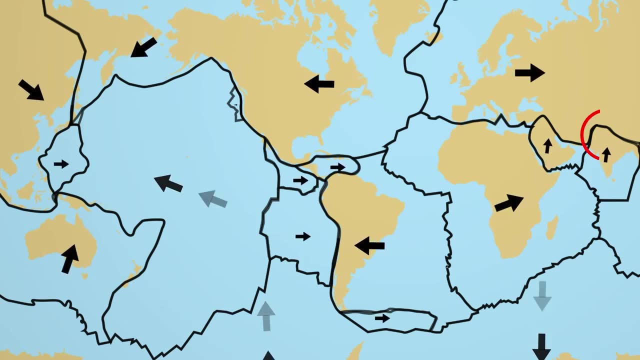 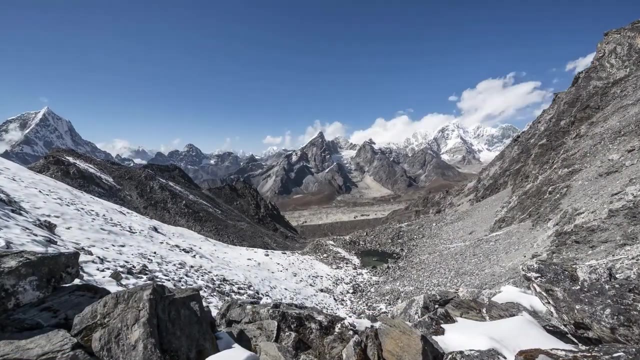 same density, They crash head-on and crumple upwards, creating what we call old mountains. You can see this is happening between tectonic plates like the Indian and Eurasian plates, where the force of the two plates colliding has created the mighty Himalayas mountain range, As you can. 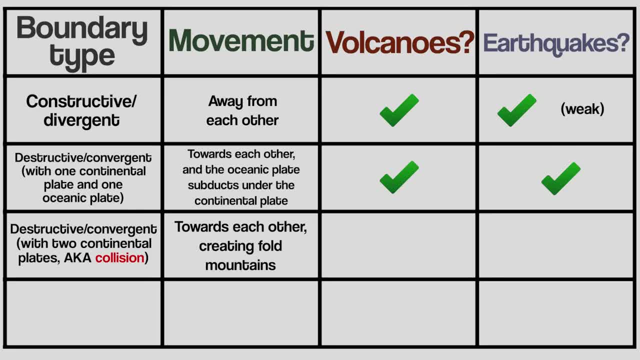 imagine. the process of forming a mountain range isn't a smooth one. The plates grind and crack and buckle upwards over millions of years and at times they get locked together and get stuck on each other. Eventually the plates build up enough energy to become unstuck. The plates jolt back into movement and an 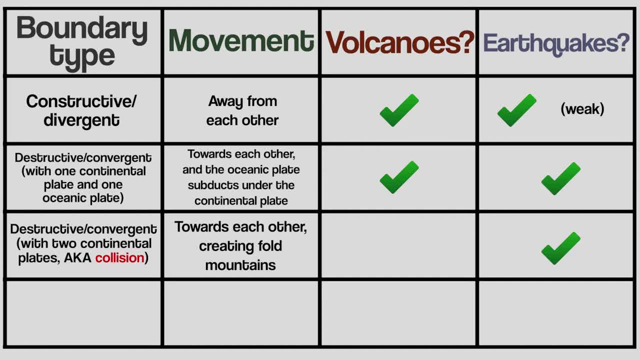 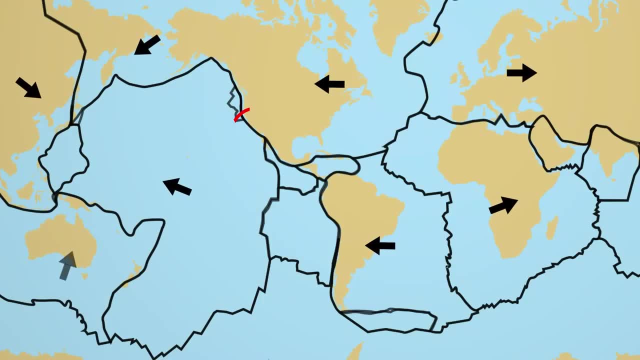 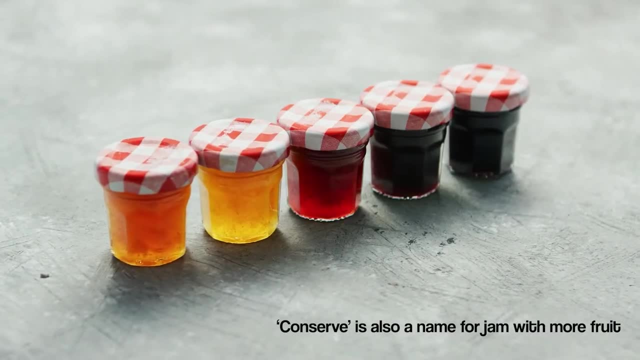 earthquake is created. Oh, and don't confuse these mountains with volcanoes. There's no magma rising up from underneath them, so you don't get any volcanic eruptions at collision boundaries. Conservative boundaries, sometimes also called transform boundaries, are so named because the tectonic plates are not being constructed or destroyed here, so it is a. 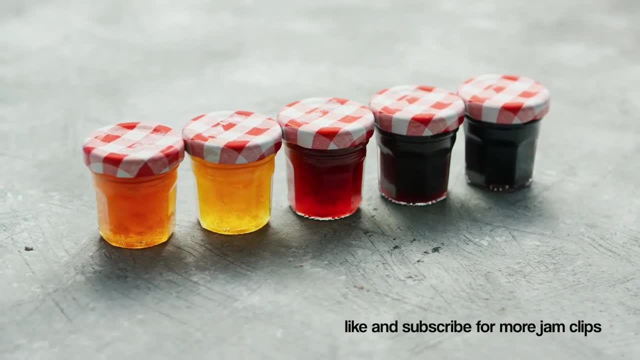 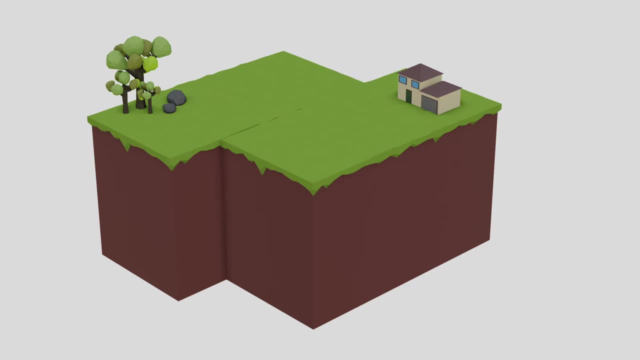 conservative boundary. The tectonic plates are not being preserved, which means to be kept the way it is. These conservative boundaries happen at places where two tectonic plates are sliding past each other, either in opposite directions or in the same direction at different speeds. The edges of the plate get stuck on each.